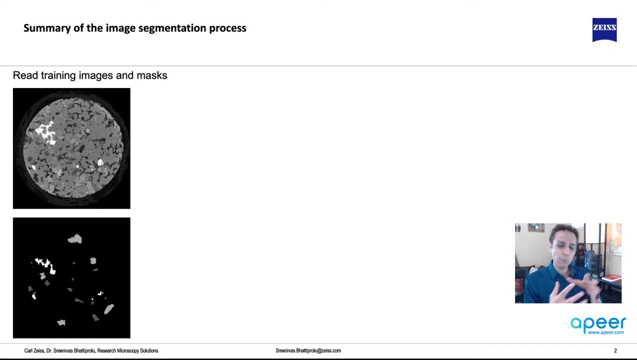 clays. So my goal is to segment a whole bunch of images that look like this, And it's a 3D volume for all of these four different regions, which means I have to provide a ground truth initially to the machine learning. This is a supervised machine learning algorithm, So I have to provide 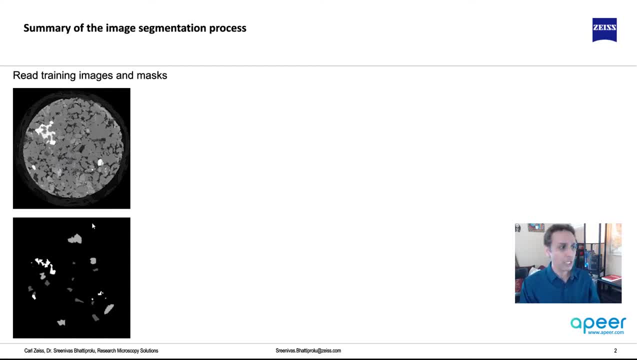 ground truth in terms of what is what. So, as you can see down here, this is a mask or a labeled image, where I labeled each of these regions in a different pixel value with a different pixel value. Okay, So here, first of all, any region that's outside that. 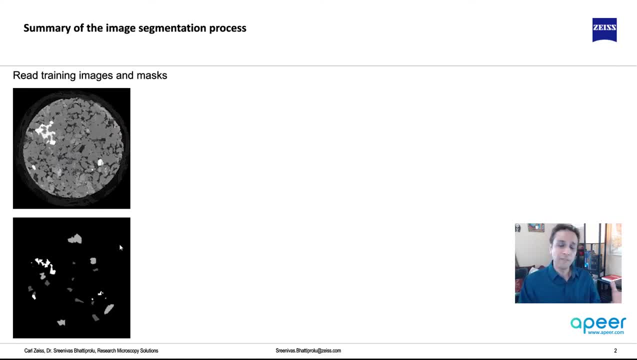 looks completely dark is a region that I did not label. For that we gave a value of zero. So every pixel value that has a zero, a value of zero. we haven't labeled it. And then value of one is the one where we did label. Two is another region. Three is another region. Three is another region. 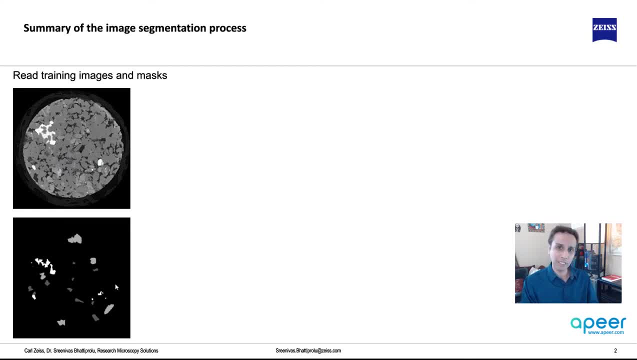 And four is another And you may have your own ways of labeling, but it doesn't matter What I recommend. if you do not have a way of labeling your images is using, appear, annotate- We'll get to that in a second. And once you have a labeled image, meaning ground truth. 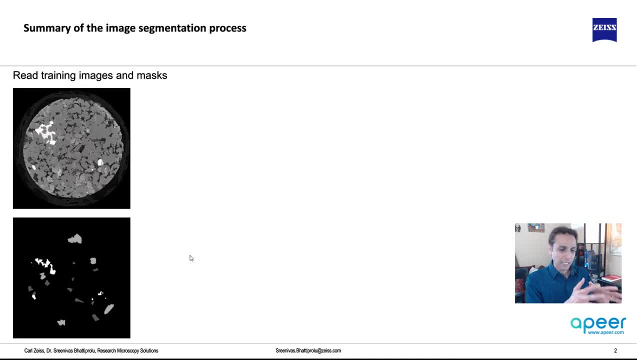 the next step is any machine learning. it takes an input, trains it okay and then gives you a model. Now, if the input is a zero, it's a model. If the input is a zero, it's a model. If the input is a zero, it's a model. 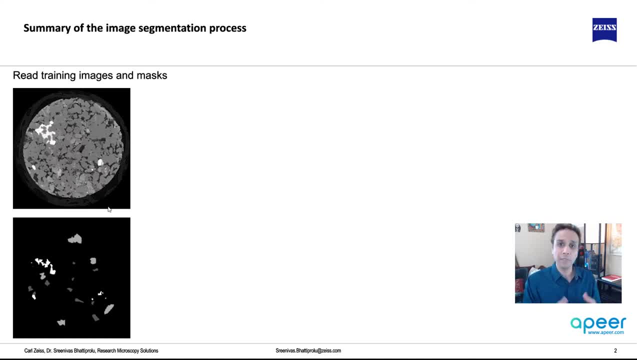 If the input is only pixel values, then we may as well do histogram segmentation. So you just use OTSU or something and then say, okay, any pixel value or multi-OTSU pixel value below a certain range, all dark pixels and so on. But that doesn't work in most cases because edges 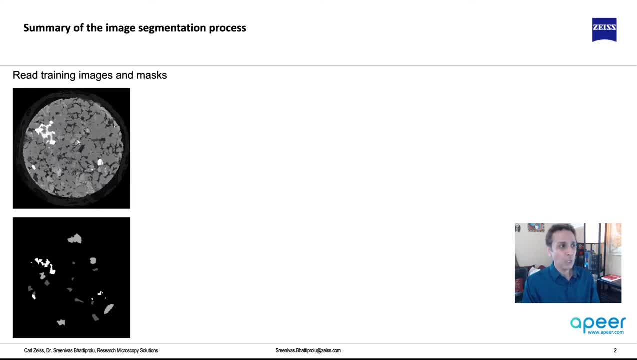 and other regions. I mean, we are using machine learning for a reason, So the best way to train a machine learning algorithm is to generate a whole bunch of features. If you're good at knowing which features actually work the best, then you can call it feature engineering, because now you're. 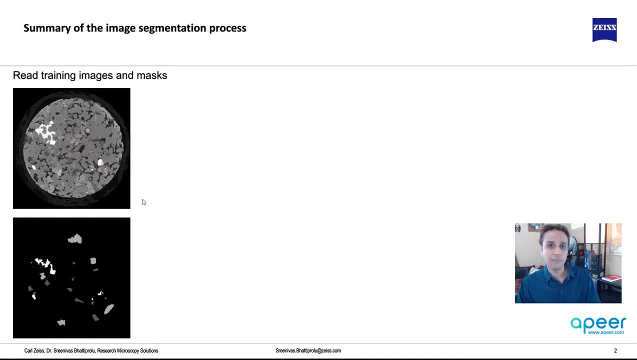 engineering features in terms of which works the best for the machine learning model. But most of the time we probably don't know what works best. So we generate 50 to 100 different types of features from this image and then feed that into the machine learning algorithm. So when I say how? 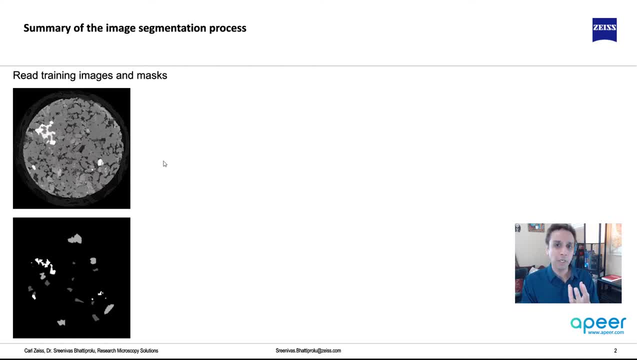 do we generate these features? this is where the term Gabor fits in. So the next thing is: these go into this feature extraction process where we apply a Gabor filter. We'll talk about what that is, Just a quick reminder, in a second. Think of this as applying different filters. I apologize. 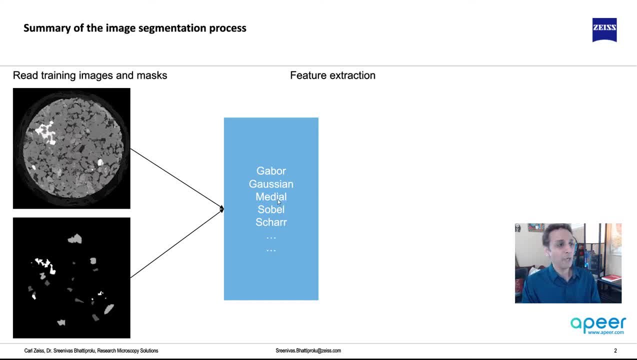 for this spelling mistake. This is supposed to be median filter. But think of applying a Gaussian filter on top of your to your raw image. What do you get? A blurred image correct, Depending on the kernel size of Gabor, of Gaussian, That filtered image. now look at pixel value. 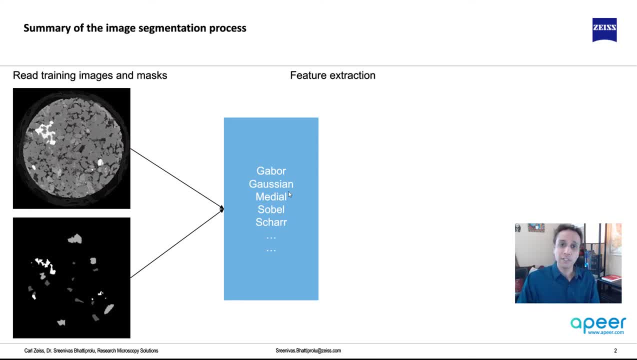 at every location, and that is your feature. So a Gaussian filtered image is one of the features that we are supplying to the machine learning algorithm. A median filtered image, a edge detected, you know, filter filtered image. So all of these, and Gabor, by its nature, generates hundreds. 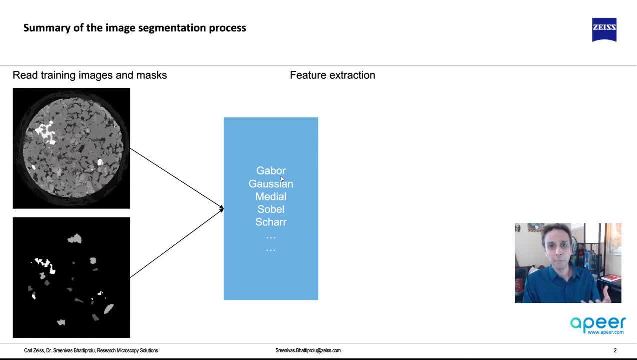 if you want you know of these responses, that makes a great feature extractor for this type of approach. Okay, so at the end of this, what you get is think of this as an Excel sheet where you have different columns. Each column represents the pixel values for a given feature image. So, for example, I have 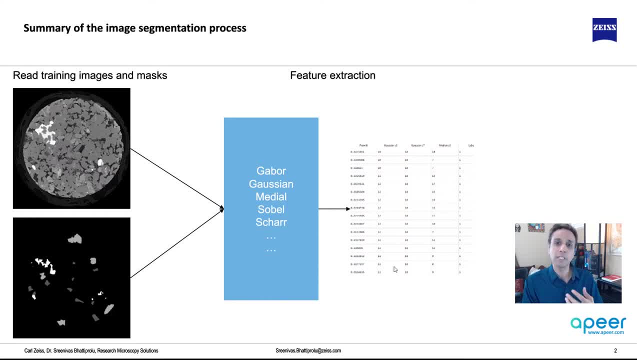 Gaussian, with a sigma value of three at every pixel. What is the pixel value? And then median filter, sigma value three, and so on, And the last column is a label. and label is again: is it zero, Is it one, two, three, four? Label is the ground truth. Okay, so I hope. 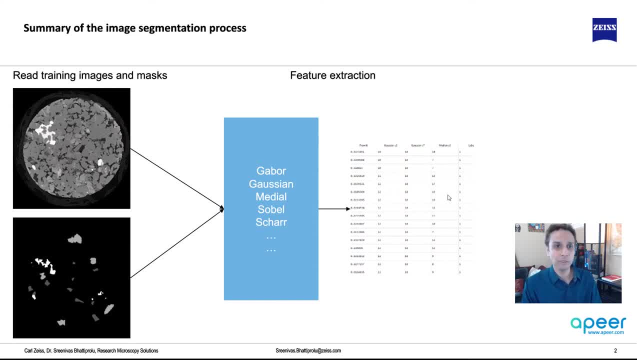 your okay so far. And then we train a machine learning algorithm by feeding a whole bunch of X values and the Y value. X values are all the features. Y is the output that we are looking for And in this case the output is the label. So for that we are going to use either random 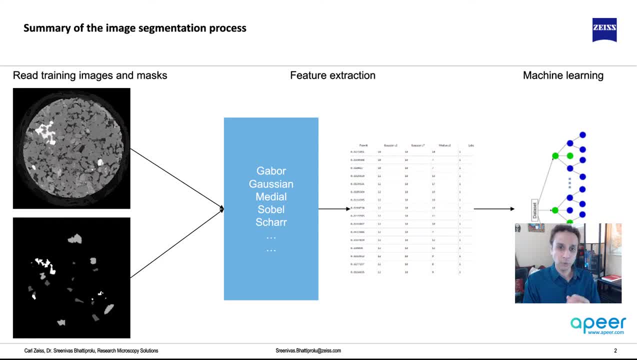 forest or support vector machine. In this case, I'm showing a pictorial representation of random forest, And I'm fully focusing on these two because these are the primary methods that most people use when it comes to machine learning, And I think these are the 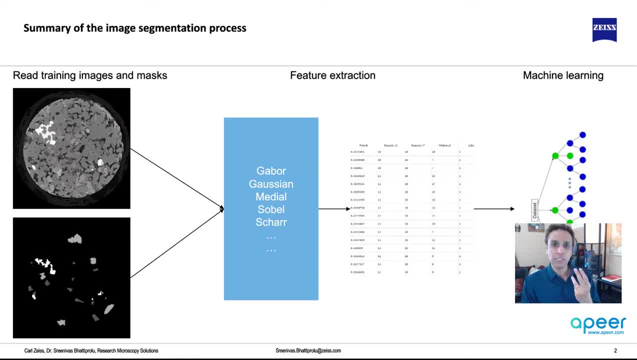 most relevant ones anyway. So just a quick reminder about the three main things that we talked about. In fact, four main things that we talked about. One is labels, The other one is features and the other one is random forest, And the last one is support vector machines. First labels: What do we? 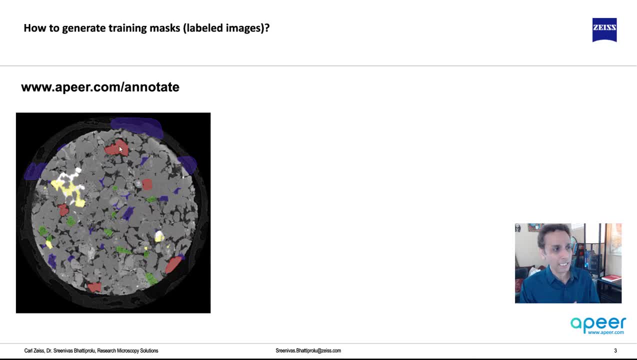 mean by labels. You take your raw image and, let's say, you paint each region of interest in different color and then assign a specific pixel value. So for all the regions we colored in purple, We are giving a value of, let's say, one and once in. 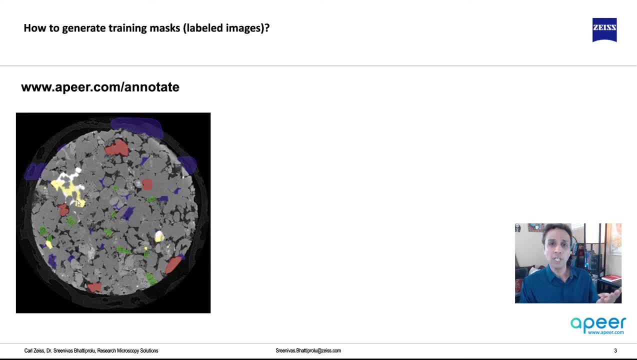 you know, red, we are giving a value of two, and then three and then four. So this is what a label is, and you can do that on Appear. If you haven't already signed up, go to appearcom- annotate to get a quick look at what we are talking about here And then, once this is done, you can just 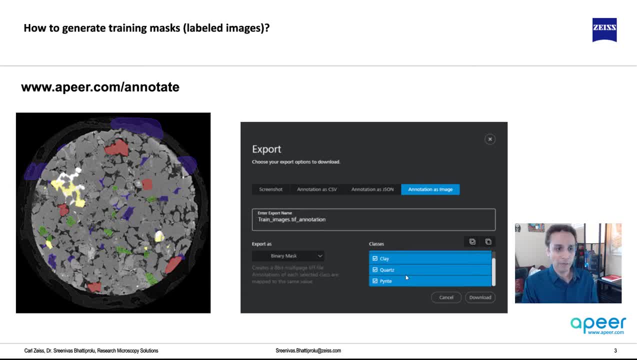 export the annotation as image and then select a binary mask and do that. And then, once we're done, we just export the annotation as image and then select the binary mask and do that. And then, once this is done, you can just export the annotation as image and then select a binary mask and do that. 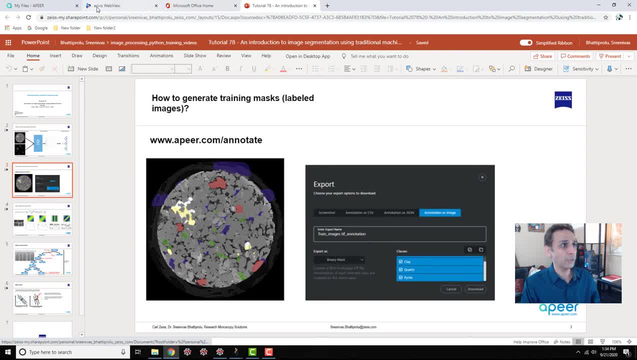 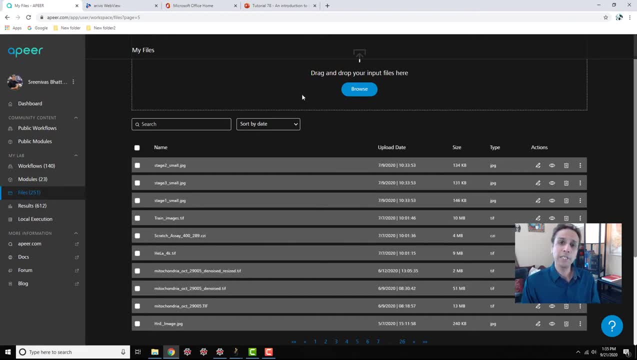 then export it. And how do we do that? Let me quickly show you the process. So, first of all, sign up for appearcom and then, under files, upload your image, And the image can be a TIFF stack or individual TIFF files. It's up to you how you want to handle this data In this example. 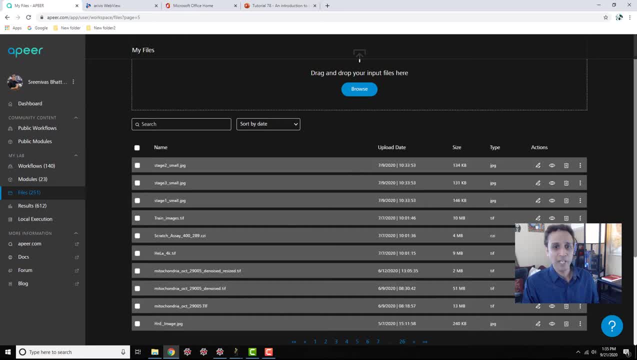 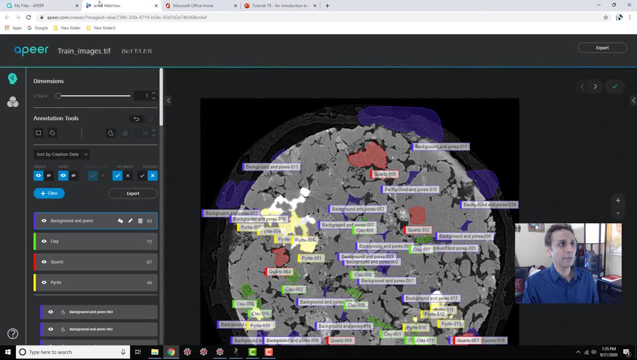 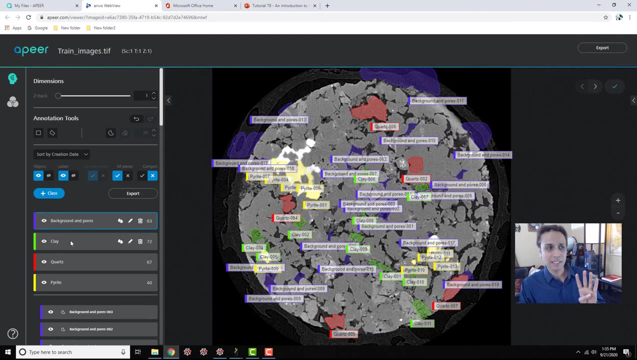 I have a TIFF stack- I called it trainimagestiff- And I click on this button that says annotate image: not the eye, but the pencil. Okay, It opens up a window like this And now you can define the classes. In this example, I defined four classes. Yeah, The background, clay quads. 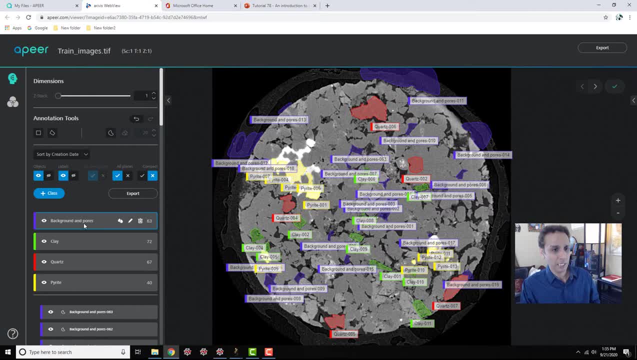 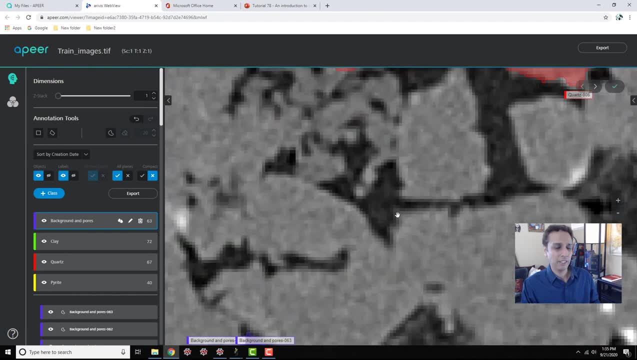 and pyrite, And you can change the colors. And for each of this, for example for background and pores, let's say this is a pore right here And I would like to label which like right here, And I just select the brush tool and then just go ahead And you can. 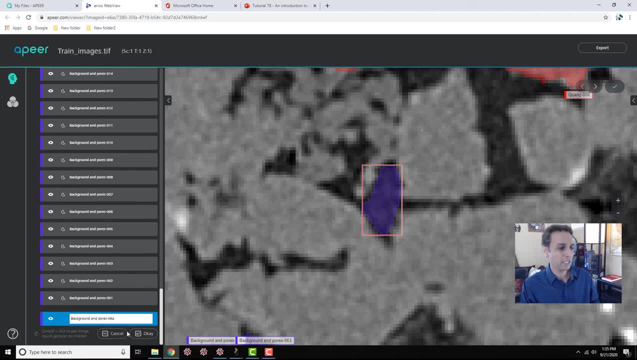 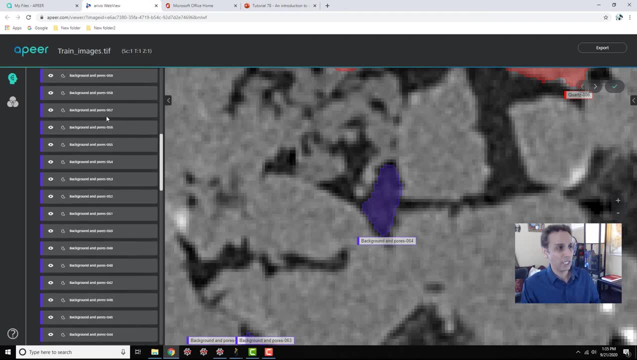 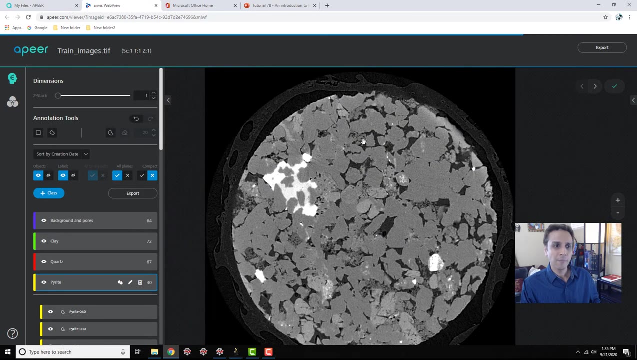 change the brush size and go ahead and paint the pixels you want, Click okay And it gets added to the other purple labeled regions. So once you're done, I mean obviously go ahead and continue for the clays and quads and pyrite, But once you're done labeling, you can actually go. 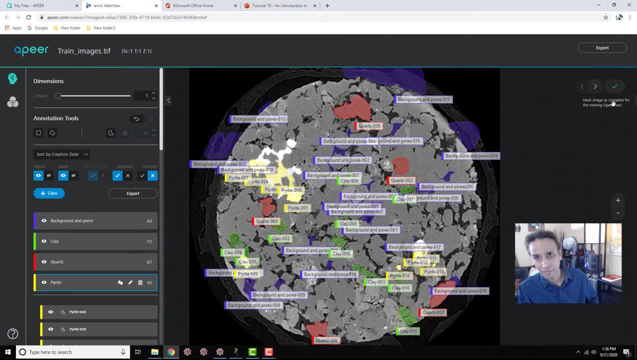 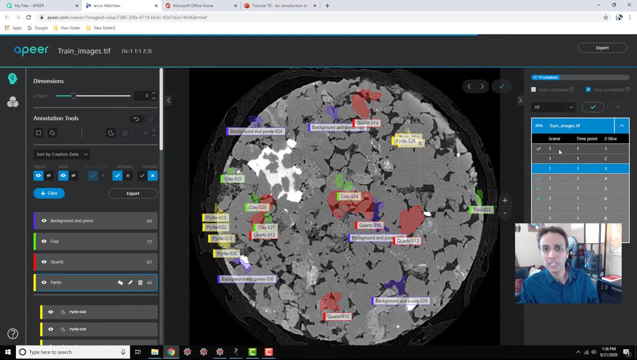 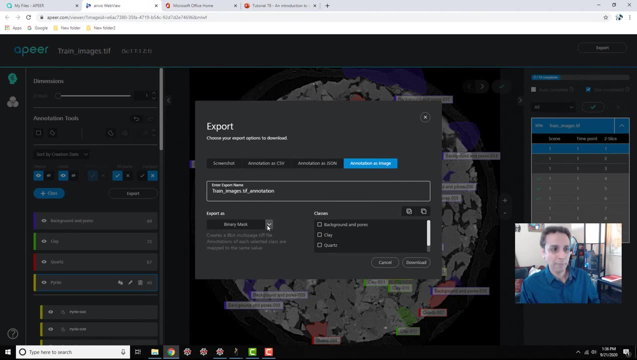 in this case, this is a. this is a, I believe, multiple images. So if I expand this, you can see this is my slice number two, slice number three and so on, And go ahead and paint these And, once you're done, export it as an image binary mask. 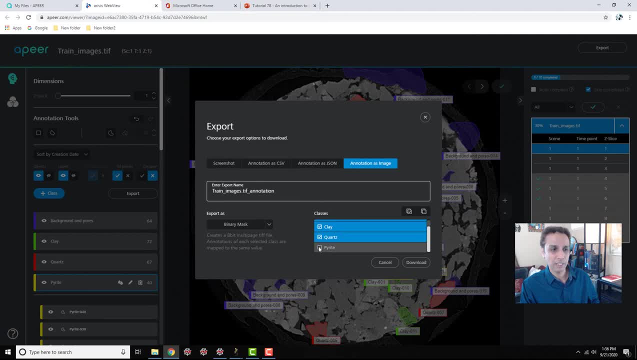 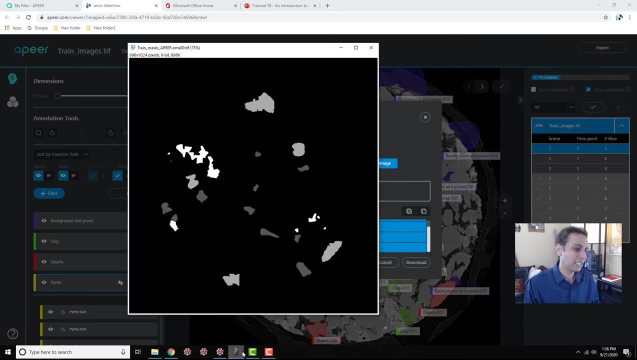 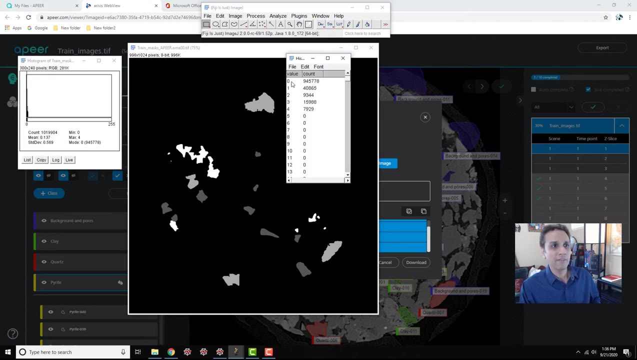 and select all of these classes that you just labeled and download. And that file would be an OME tip file. So if I open it it looks somewhat like this And if you look at the histogram you should see that the pixel values are 0,, 1,, 2,, 3,, 4, 0.. For all the regions where 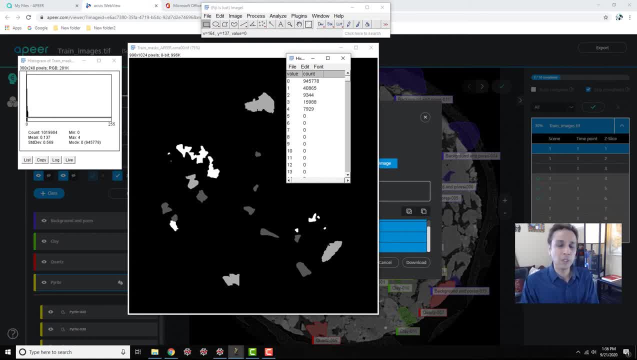 I haven't labeled. we don't want that to be part of our training, because they don't correspond to anything. So we are going to drop all the pixels with a value of 0. The only relevant ones for us are 1,, 2,, 3, 4.. Okay, This is the process. if you use a Pierce annotate tool, which I highly. 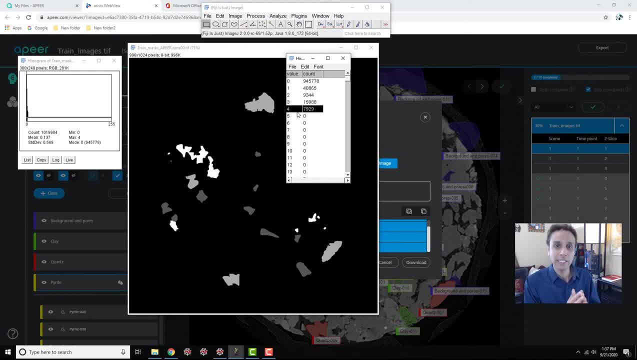 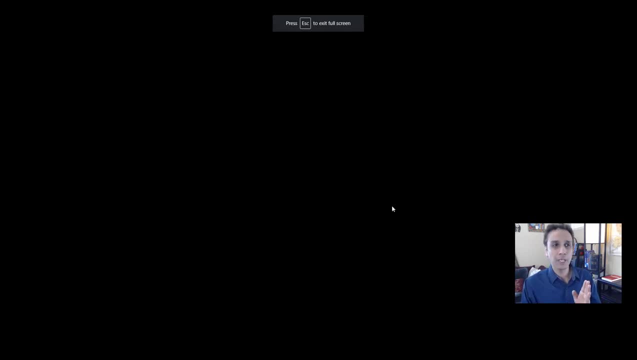 recommend. If you use any other tool to do your labeling, fine, It's still okay, As long as you know that. okay, you have unique pixels, pixel values corresponding to a specific region. So let's get back to our discussion here. So so far, you know how to export your labels. Now let's 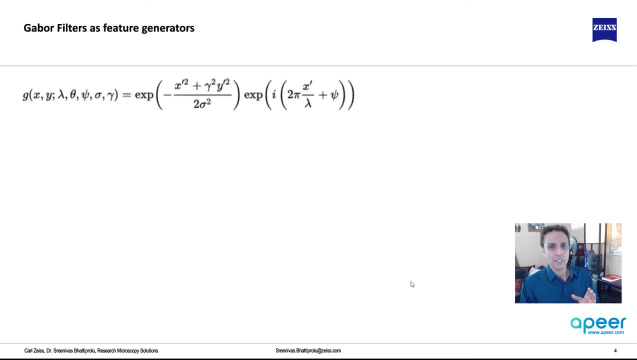 look at Gabor filters, and Gabor filter is a convolutional filter and it's got multiple terms and it's a function of wavelength- theta, phase, sigma and gamma- And by changing these values you can generate infinite number of filters. Obviously, the system cannot handle. 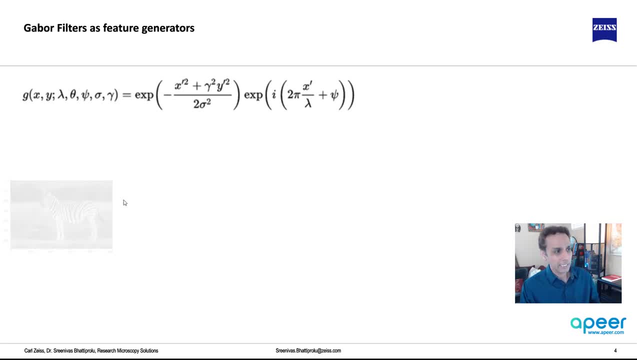 infinite numbers, So you change these appropriately. But in this example you can see I have a zebra Again. I covered this in our video, exclusively about Gabor filters, So I'm just giving you the highlight summary here. So by defining theta as 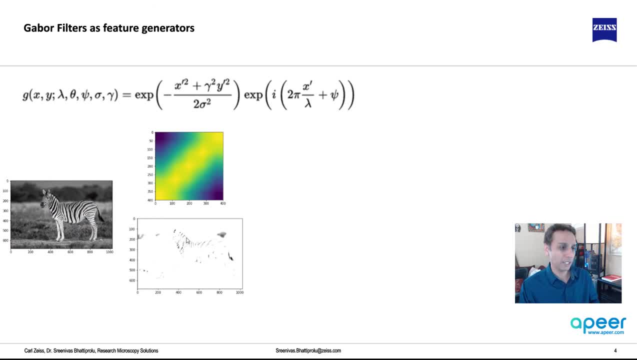 45 degrees. in this case, we are detecting all the regions that are aligned in a way about 45 degrees to this filter. This is just a bandpass filter, So we're just looking at all the regions that goes through this specific filter. Now, by changing another parameter, you can just see how. 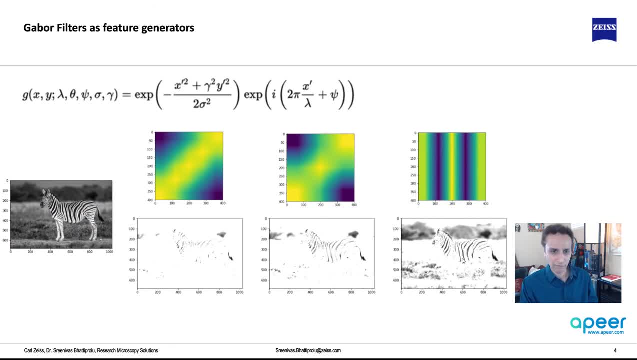 I move this vertically, So I'm seeing a lot of vertical bands and so on. So you can see how, by changing the theta, the phase and the gamma, which is, you know, the, the, how much you know. 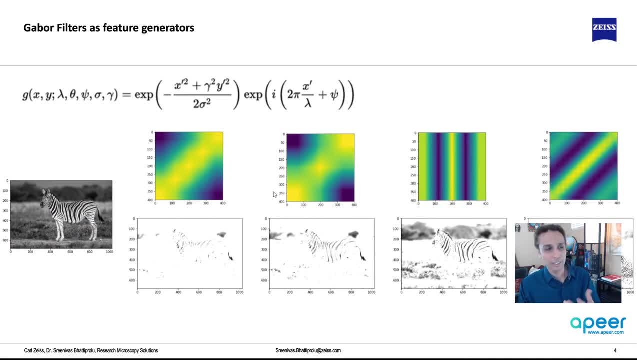 is it? how small or big is the aspect ratio? is the term I was looking for, Sorry, And so on. you can. by changing these, you can actually detect different types of features. So just imagine just extracting 50 different features like these type of images. 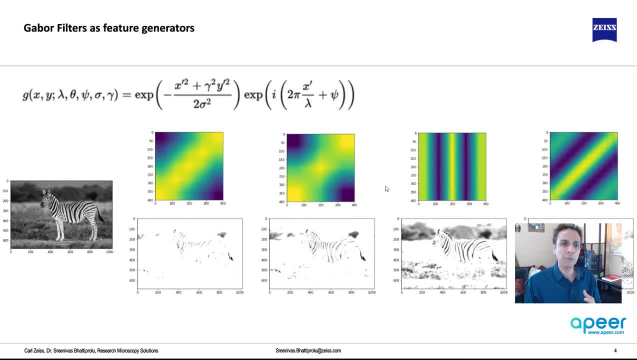 By applying these digital filters. this is almost similar to now we are getting into deep learning, where it generates these different levels of convolutional filters. except in this case, our filtered images are all static Once we filter them. that's it. That's our feature vectors. 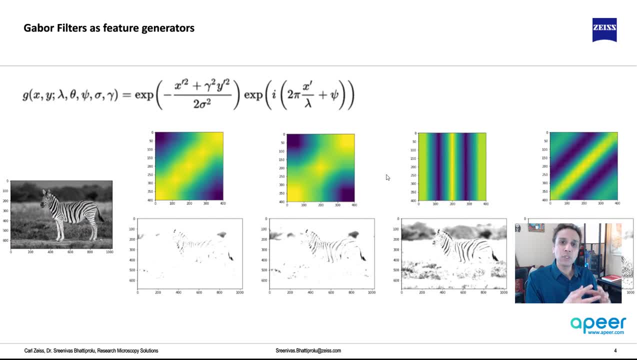 in deep machine learning, Typically the convolutional filters. they are trained. You say, okay, this is my initial set of features, And then it does the training and then comes back in the next deep pocket. It's like, okay, so these filters are all static, So we're going to filter. 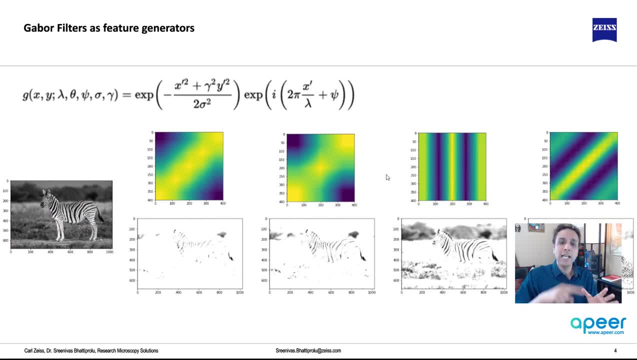 filters are working, but then these are not. So let's change the weights a little bit And then it keeps changing these weights until they converge, And then you can use that, in fact, as a feature generator here, but that's a different discussion. So that's Gabor and 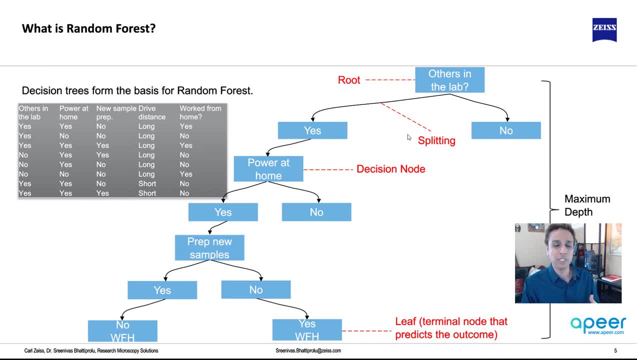 random forest. I hope you again watch this video. Random forest is basically a bunch of trees that are ensembled together and each tree, or a decision tree, is making a decision. It's very simple. So a decision tree is you start with. okay, shall I go out and play? Well, is it cold or is it hot? 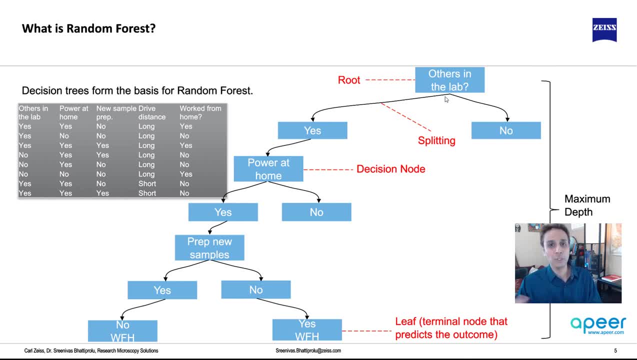 If it is too cold, okay, I'm not going to play. If it is too hot, I'm not going to play. Okay. If it is rainy, I'm not going to play. If it is not rainy, I am going to play, Okay, If it is not rainy. and 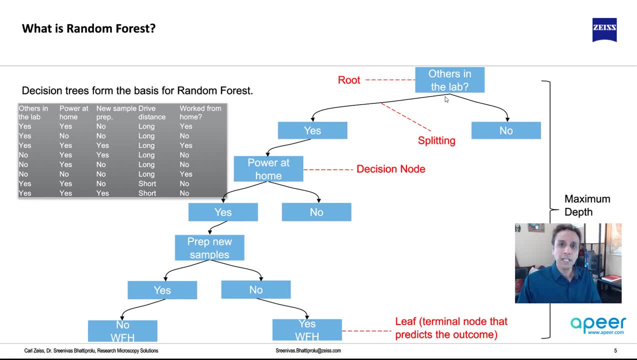 then comes down. So you're breaking it down into individual nodes And at the end of it you get a decision: Okay, Shall I play or shall I not play. And then you get a decision: Okay, Shall I play or shall I not play. So in this case, is it a pixel one or a pixel two, or a pixel three or a pixel?